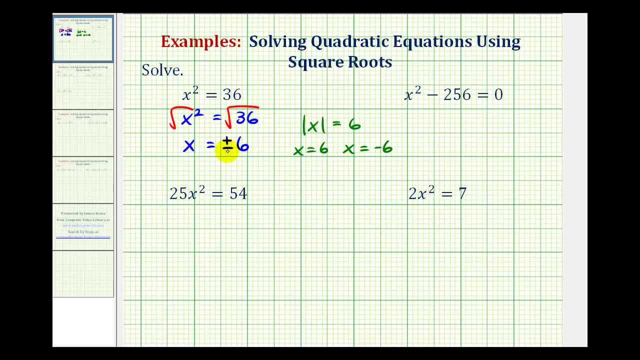 But if we were to solve this equation, we would have x equals positive 6 or x equals negative 6.. It's not often shown this way, But this is the real reason why we have to include a plus or minus sign when taking the square root. 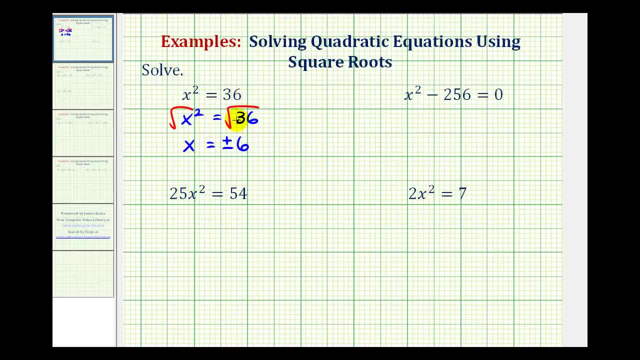 of both sides of an equation. And one more thing to mention here, because our two solutions are real and rational. we actually could have solved this quadratic equation by saying it equal to 0 and factoring, But this video is going to focus on using square roots to solve these types of equations. 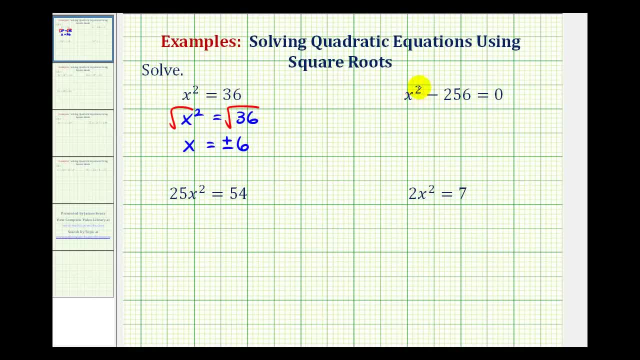 Looking at our second equation, we want to isolate x squared, so we need to start by adding 256 to both sides of the equation, So we'd have x squared. this would be 0, equals 256,. and now, because x squared is a perfect square, 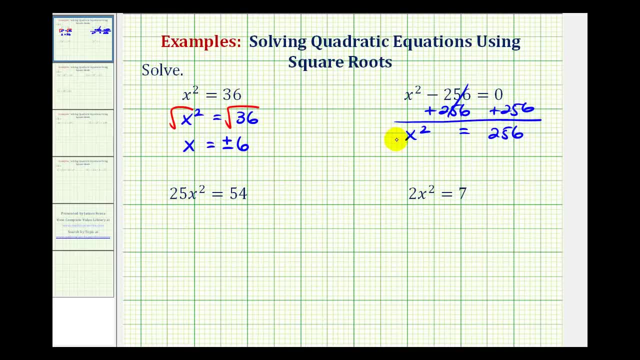 we can solve this for x by taking the square root of both sides of the equation, And when doing so, this time I'll include the plus or minus sign here. So the square root of x squared is: x equals plus or minus. 256 is actually a perfect square. 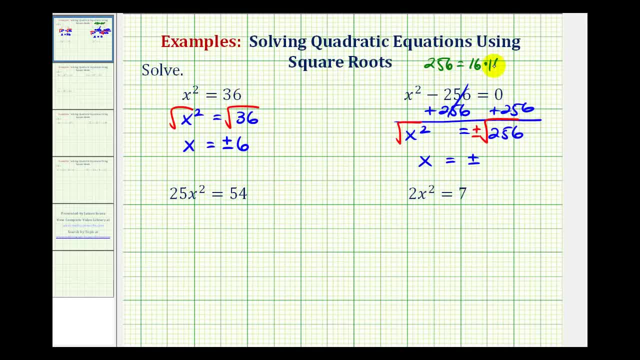 256 is equal to 16 times 16, so the square root of 256 is equal to 16.. So our two solutions are x equals 16 or x equals negative 16.. In our next equation we want to solve this for x squared, so we need to divide both sides. 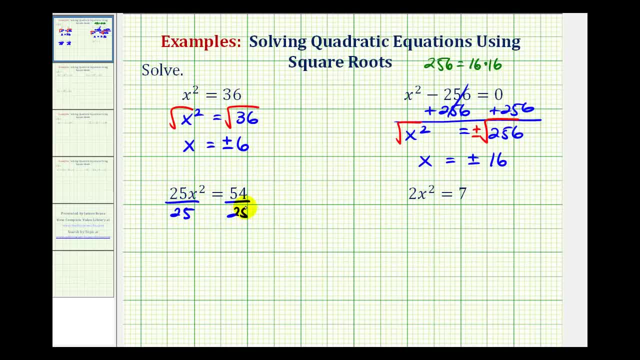 of the equation by 25.. So we'd have x squared. this would be minus, and then we'd have x squared. we'd have x squared equals 54 over 25.. And now to solve this for x, we'll take the square root of both sides of the equation. 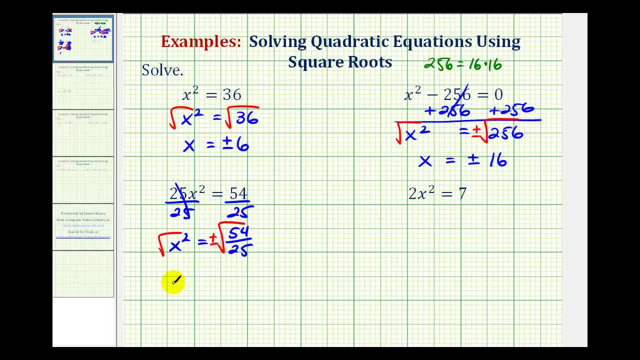 add our plus or minus sign here, So we have x equals. we can rewrite this as: plus or minus, the square root of 54 divided by the square root of 25, and notice that 25 is a perfect square. So the denominator simplifies to the square root of 25 or 5.. 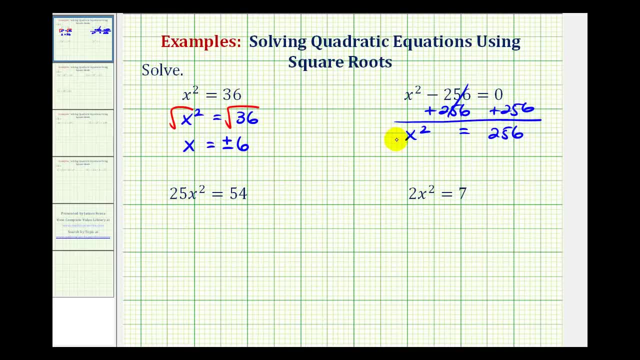 we can solve this for x by taking the square root of both sides of the equation, And when doing so, this time I'll include the plus or minus sign here. So the square root of x squared is: x equals plus or minus. 256 is actually a perfect square. 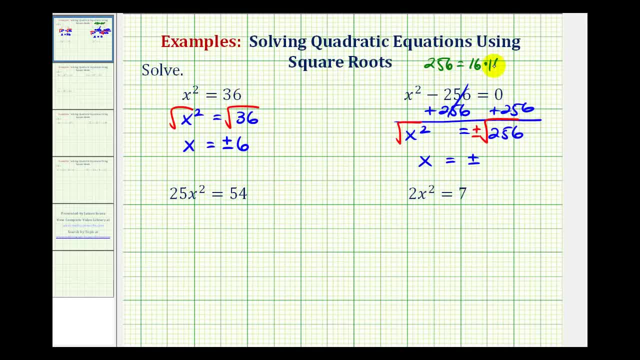 256 is equal to 16 times 16,, so the square root of 256 is equal to 16.. So our two solutions are x equals 16, or x equals negative 16.. In our next equation we want to solve this for x squared, so we need to divide both sides. 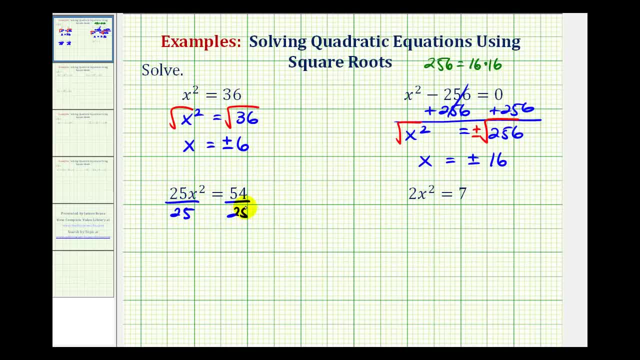 of the equation by 25.. So we'd have x squared, this would be 0, equals 16.. We'd have x squared equals 54 over 25.. And now to solve this for x, we'll take the square root of both sides of the equation. 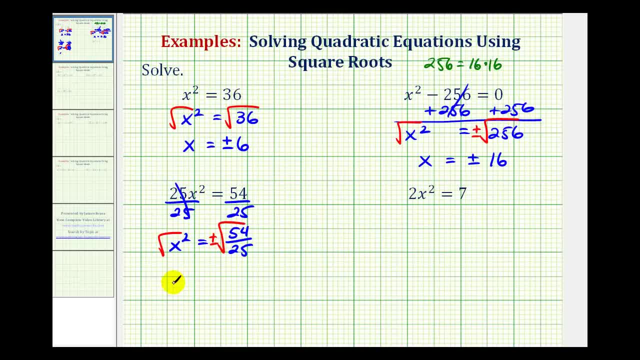 add our plus or minus sign here, So we have x equals. we can rewrite this as: plus or minus, the square root of 54 divided by the square root of 25, and notice that 25 is a perfect square. So the denominator simplifies to the square root of 25 or 5.. 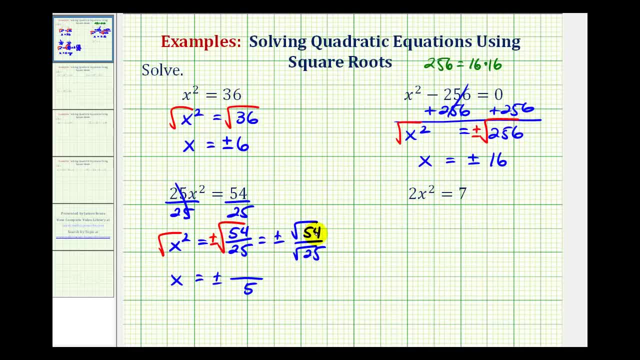 Fifty-four is not a perfect square but it does contain perfect square factors. so this will simplify. Fifty-four is equal to 9 times 6, and 9 is a perfect square. so this simplifies to: x equals plus or minus 3, square root 6, the square root of 9 is equal to 3, divided by 5.. 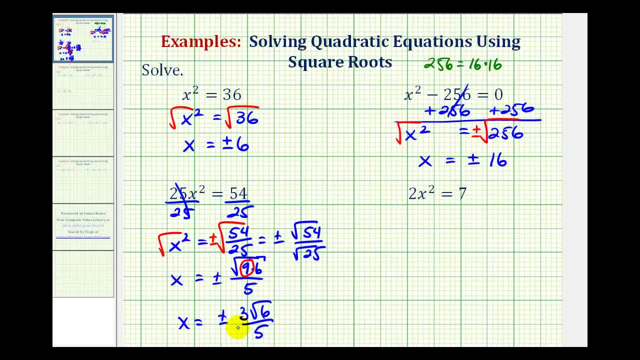 And here because we have two real, irrational solutions. this tells us that we could not have solved this equation by factoring. And for our last example, we'll solve this equation for x squared by dividing both sides by 2.. So we have x squared equals 7 halves. and now again to solve this for x. 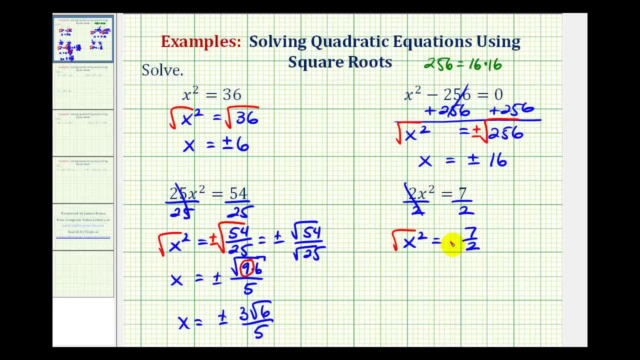 we'll take the square root of both sides of the equation, include the plus or minus sign On the right. so the square root of x squared is x, and again we can write this as plus or minus the square root of 7, divided by the square root of 2..